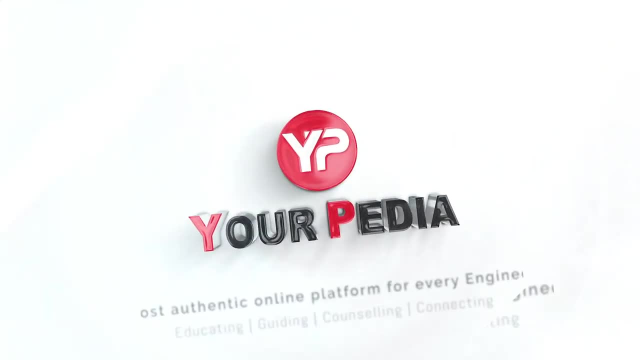 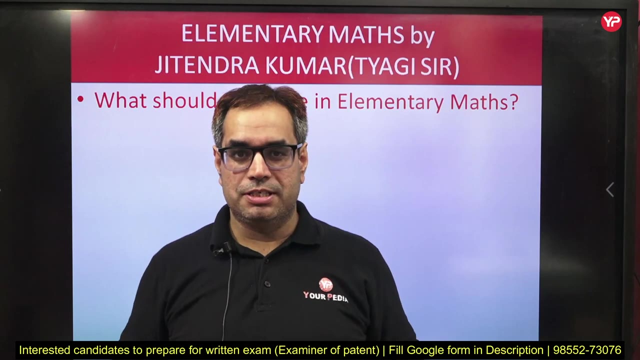 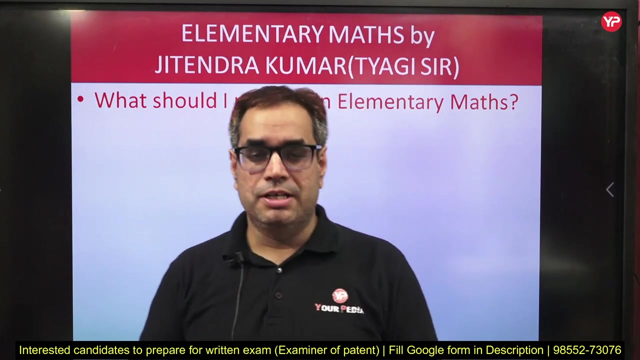 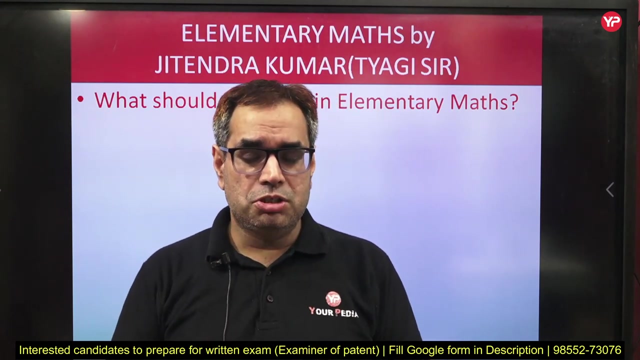 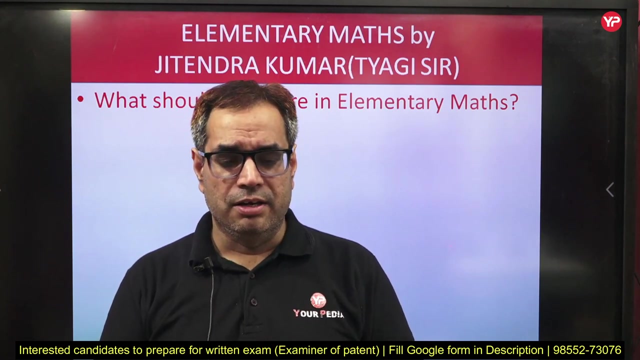 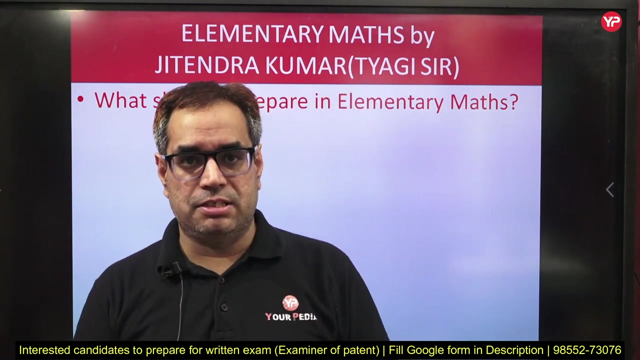 Hello students, welcome to Europe Education. I am Jitendra Ktyagi. So as all of you are preparing for your CGPDM examination, so students actually are confused for their prelims preparation as well as for mains preparation, And the most common confusion among students is regarding the syllabus of elementary mathematics. Students are not aware about syllabus, what topics they have to prepare for elementary mathematics in their main examination syllabus. 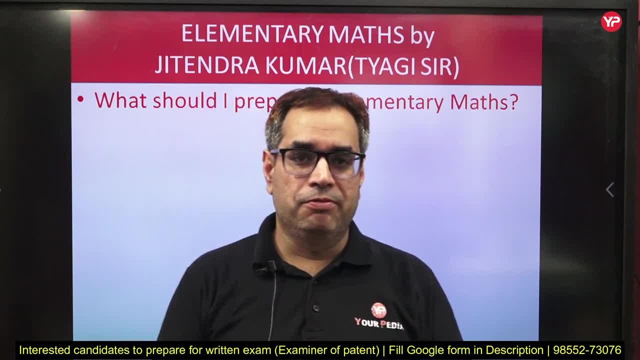 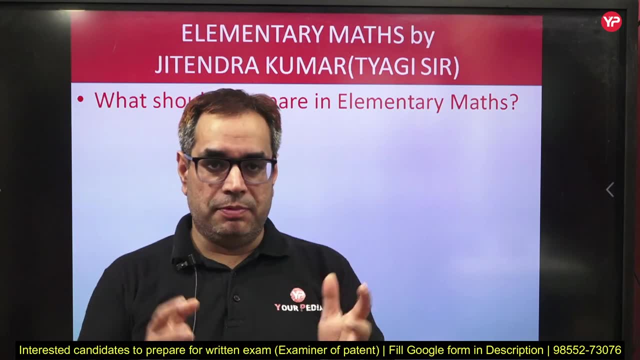 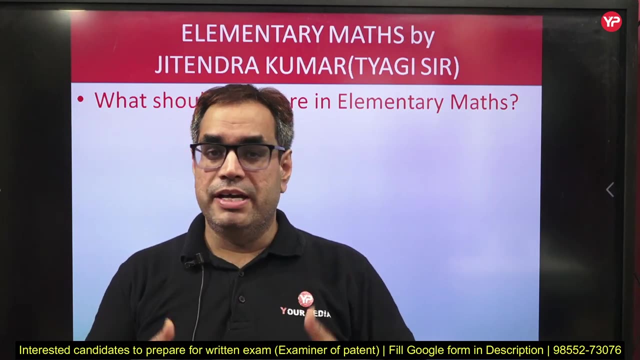 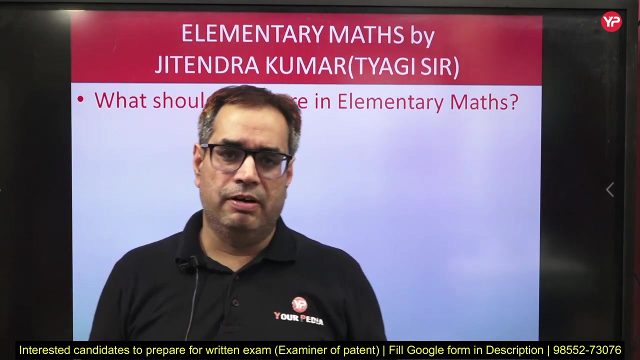 So in this video I will give you detailed information regarding the syllabus of elementary mathematics, What topics, what individual chapters, topics, concepts you have to prepare for the elementary mathematics section in your main examination, Because if prelims they conduct next month, suppose, then within one month we hope that they may conduct this main examination also. 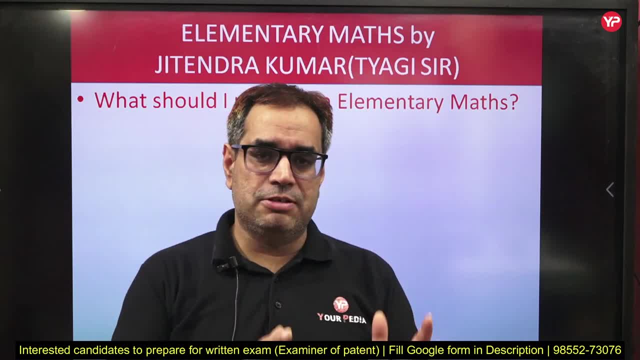 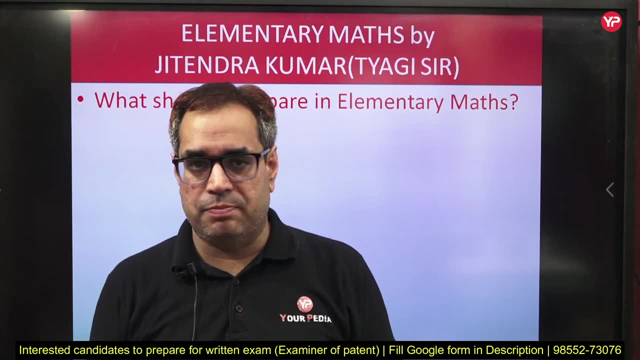 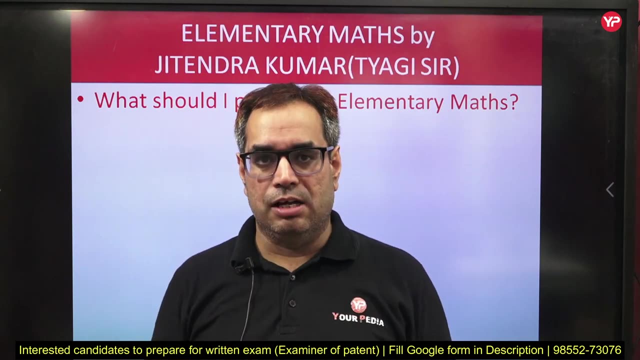 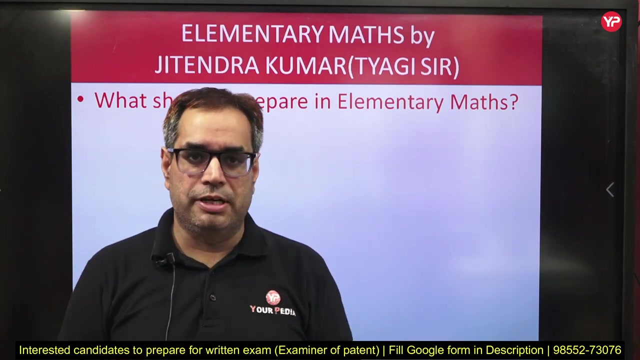 So now it is the time to prepare for both prelims as well as main examination simultaneously, Because earlier also most of the students have prepared seriously for prelims paper. So you have preparation for prelims. So along with prelims, start preparing for the main examination also. Like we have started conducting different classes on elementary mathematics of our enrolled students, So other students also should start preparing for elementary mathematics. 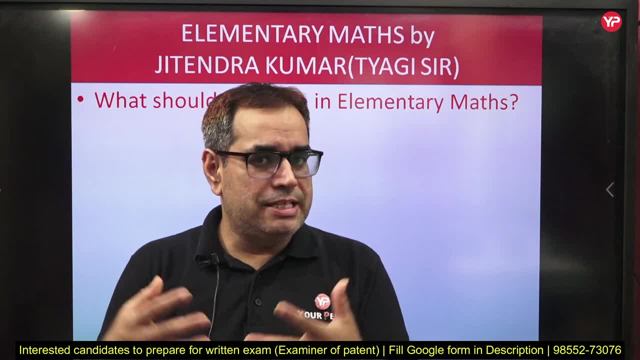 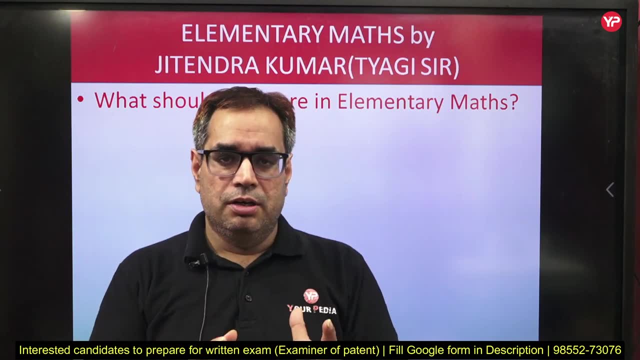 Because this elementary mathematics is containing many chapters that are common with the aptitude section also. So combinedly you can prepare for your aptitude for prelims as well as general aptitude for main examination and elementary mathematics. okay, it is a collective preparation for all these papers. 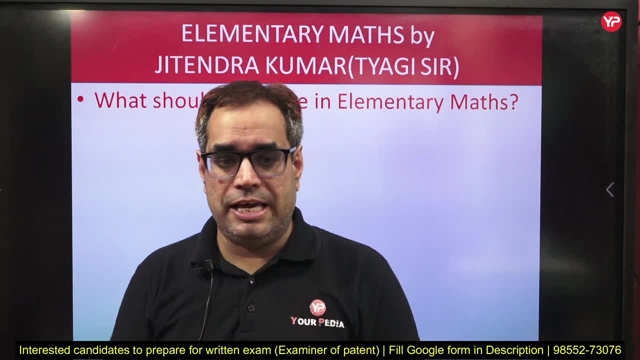 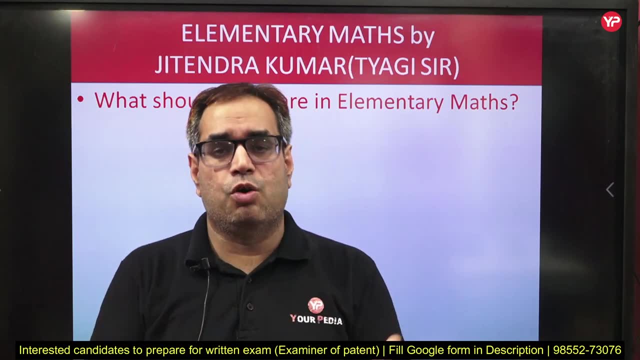 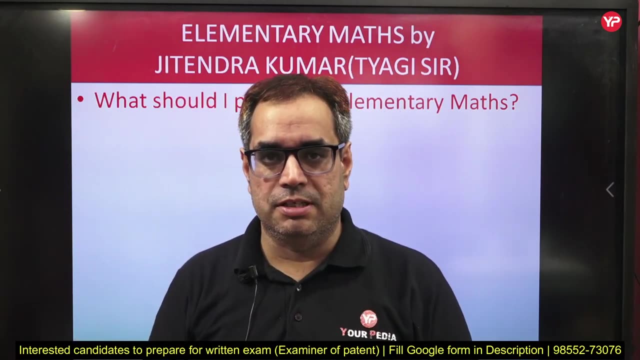 so if we add all the questions like in a previous paper, we have aptitude questions in main examination. so so many questions are there from this topic only. okay, so in detail we will discuss one by one what topics you have to prepare for this examination. okay, so let us see. 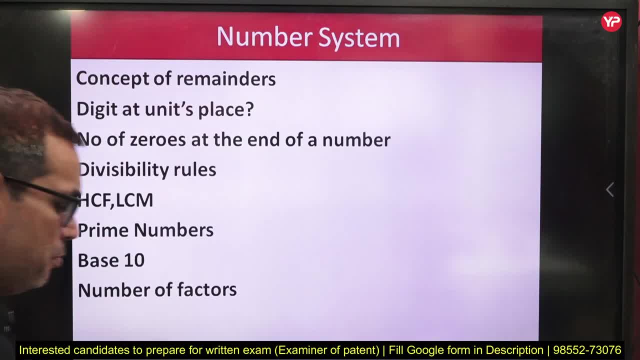 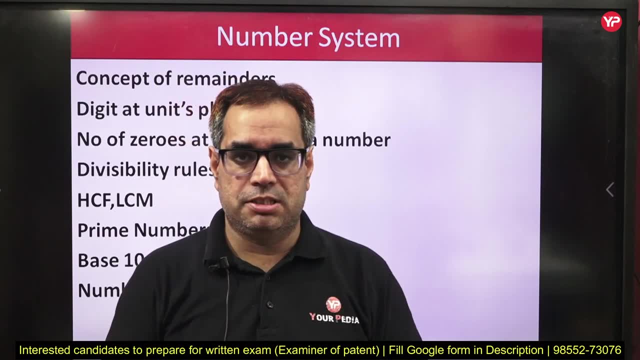 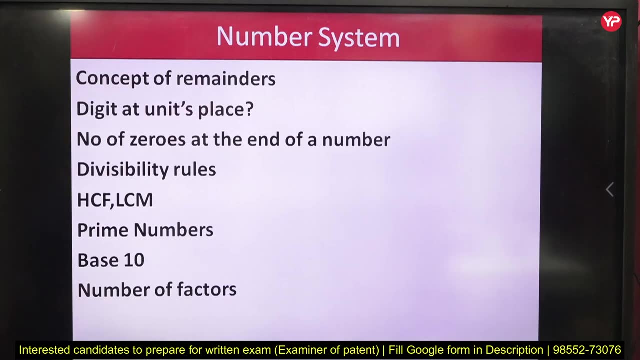 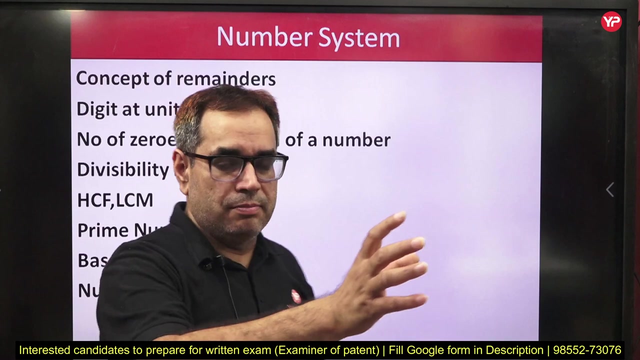 first of all, the most important chapter for elementary mathematics is number system. okay, you have to prepare number system seriously. and what are the most important points in number system which you should strictly prepare, all of you, okay. so first one is concept of remainders. you know, if this number is divided by this number, what is the remainder? such questions you have to prepare. 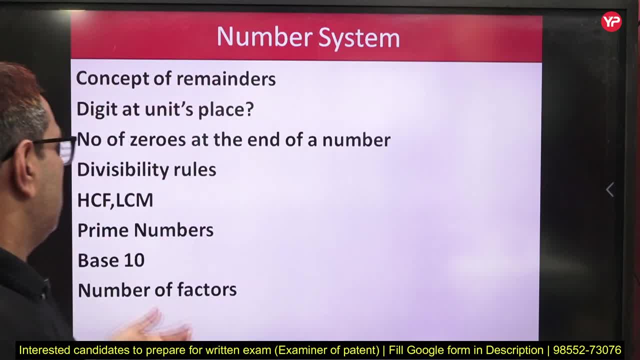 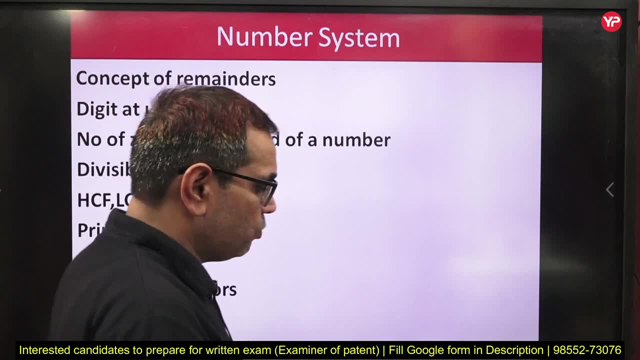 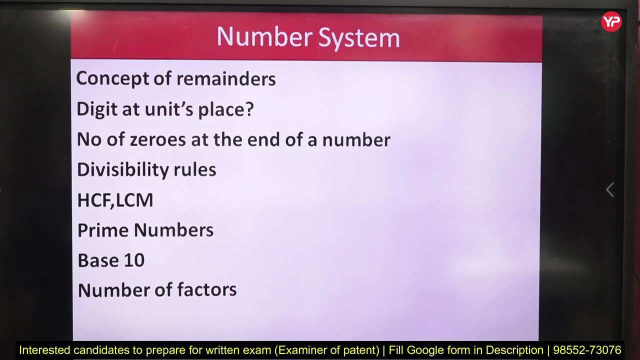 most probably you will get question 14 from this topic. ok, and digit at the unit place of a number. that is also very, very important. they will give you some number and they will ask: what is the digit at the unit place, or ones place, of that number? ok, so this is also to be prepared now. number of zeroes at the 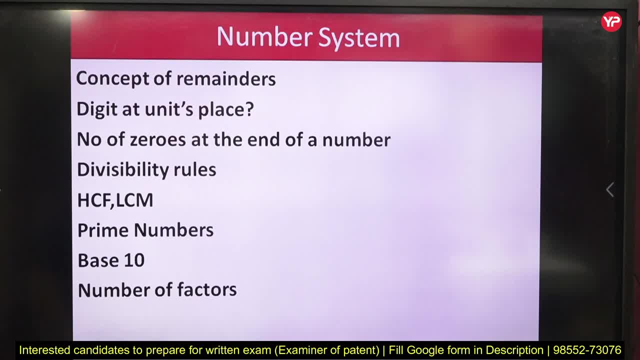 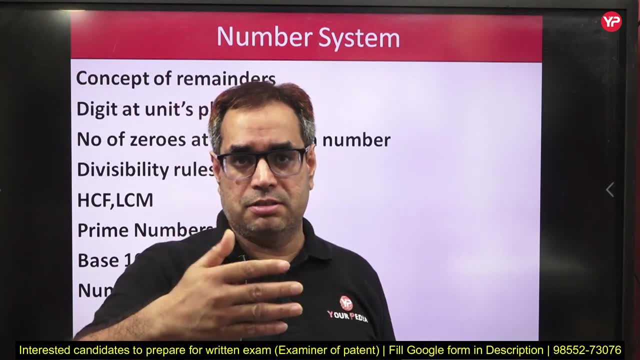 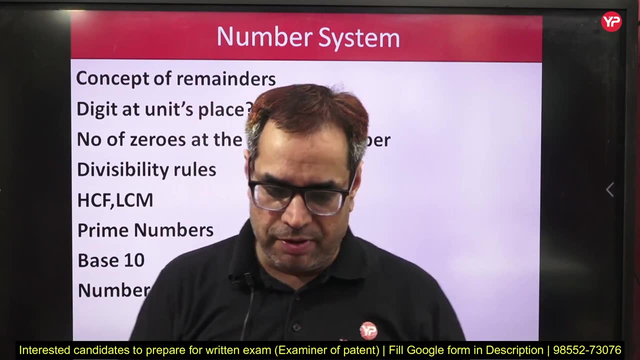 end of a number. this is also important concept. you should also prepare all the divisibility rules ok, like when a number is divisible by 3 or 4 or 5 or 6 or 9 or 8 or 10 or 11. all these basic divisibility rules you have to prepare, ok, and after that we have SCF, LCF. 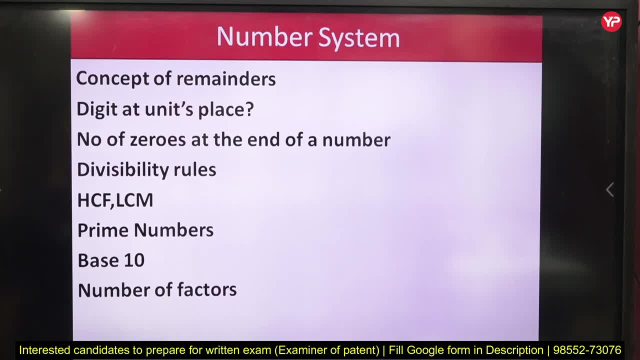 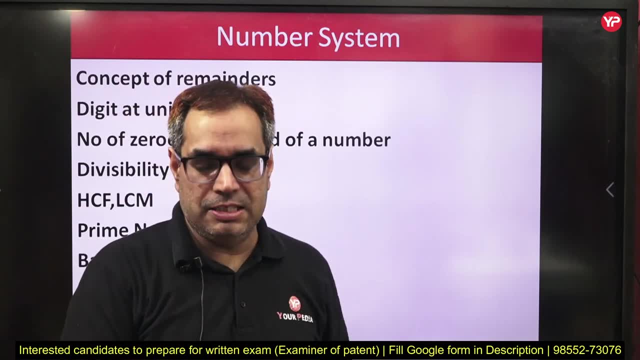 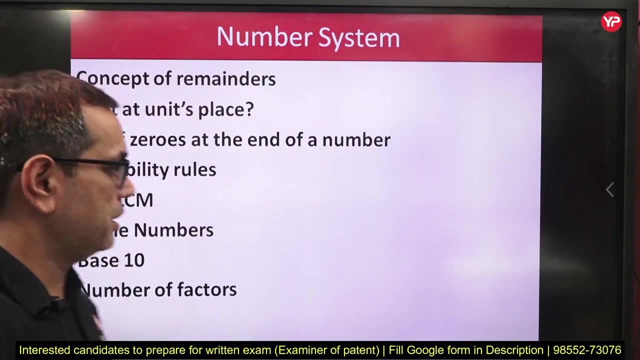 that is most important. ok, SCF and LCM. so you should prepare calculation of SCF, LCM, their relationship. ok, and different variety of questions. we have like in our classes we study many different OPEX related to SCF, LCM, all those you have to prepare for this exam. ok, then prime number. 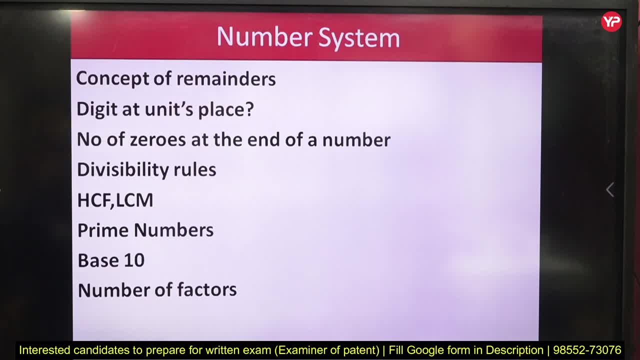 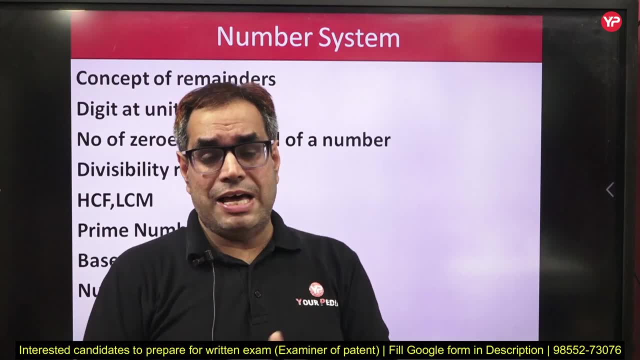 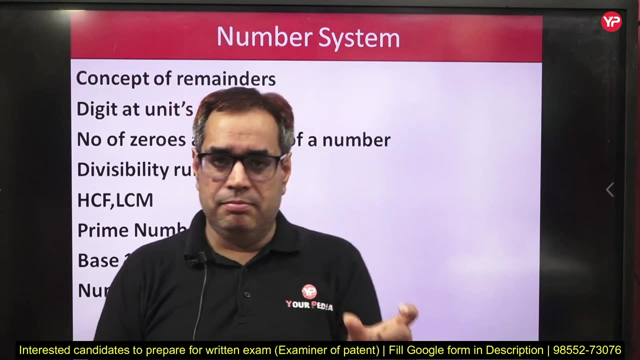 so what are different prime numbers? their identification is also important. now, base 10. you know the numbers with which we deal in our daily life. those are decimal numbers. they have base 10, ok. so such question: like a number, we have a number, ok, and if we reverse? 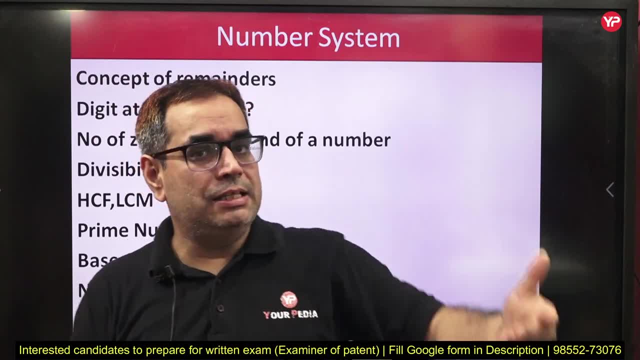 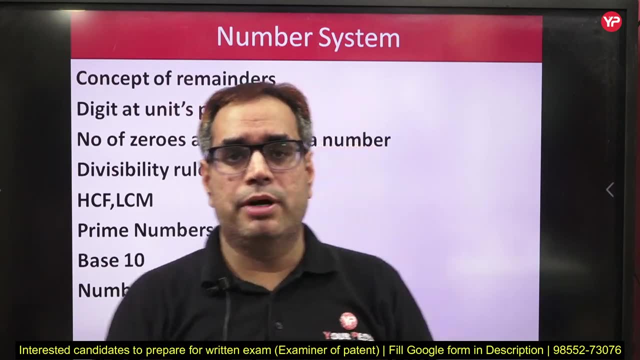 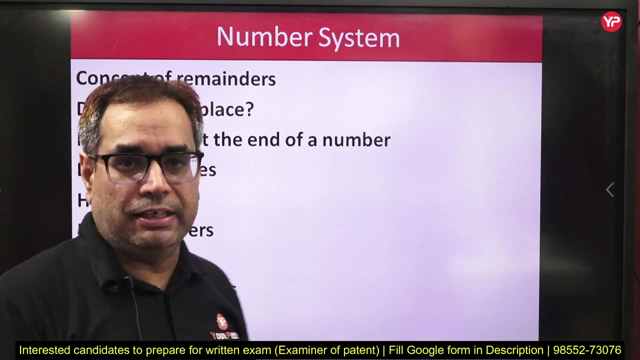 the digit of the number. the new number obtained is 20 more than the previous number. so this kind of question, which are based on the base of the number, ok, so these are also important for your examination. and then factors, ok, number of factors, number of odd factors, number of even factors, all this kind of questions are important in number. 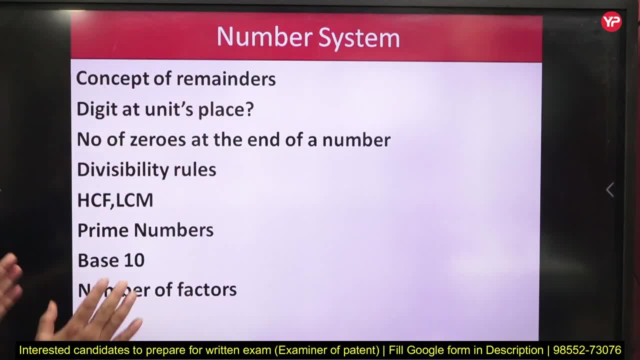 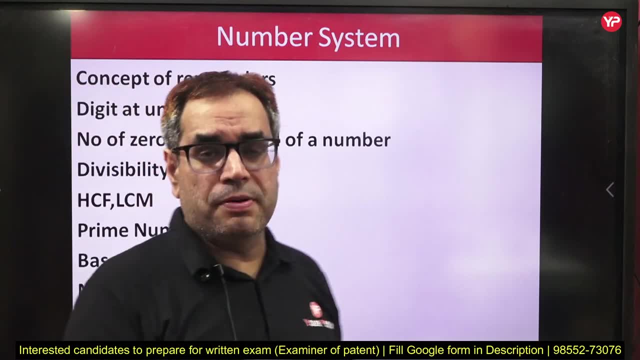 system and these questions are strictly in the syllabus of elementary mathematics. you will get questions in elementary mathematics from these topics also in your prelims paper. you may get questions And again the subject is going to be different from these topics. ok, so that is why it is a 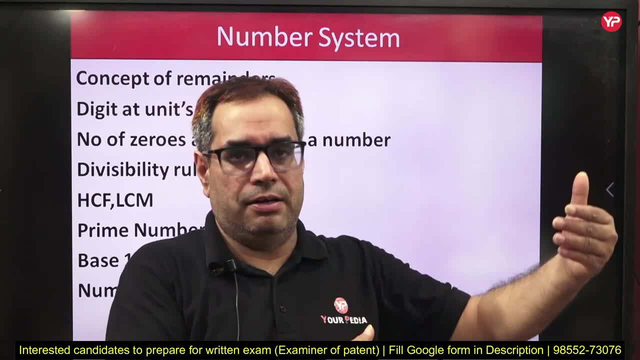 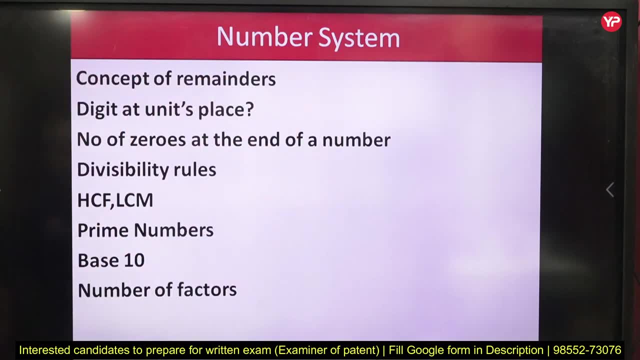 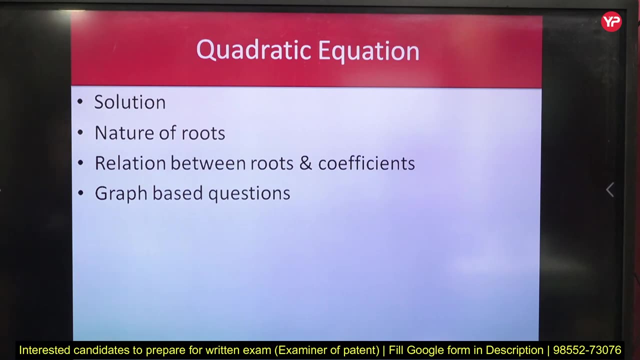 collectively. you have to prepare all the topics. it is not different that you are going to differently prepare for this. All the topics are mixed with each other. ok, so this is number system which you have to prepare for elementary mathematics and also for prelims paper. now quadratic equation. so 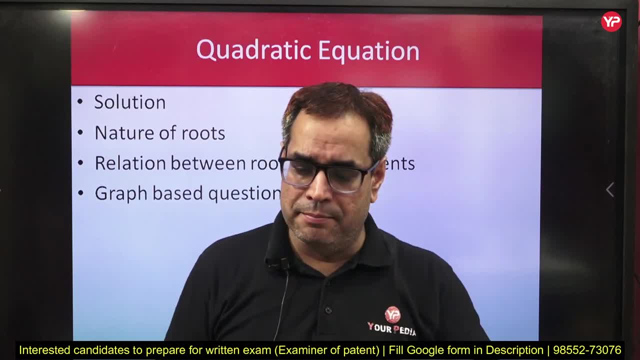 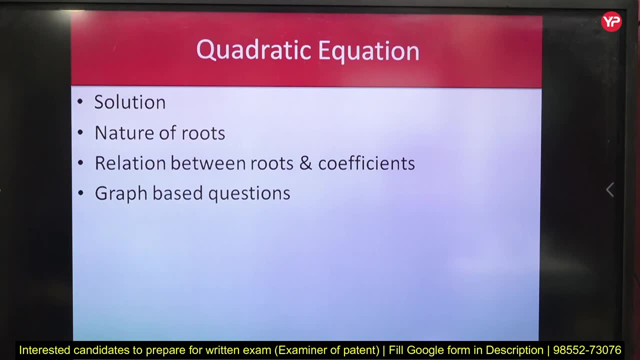 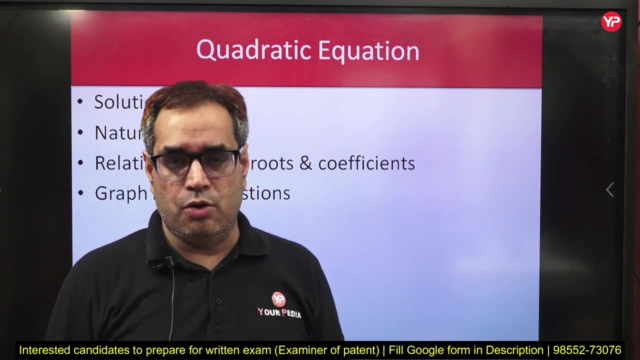 very simple chapter, is there quadratic equation, but important for your exam, ok, so in quadratic equation you should know how to solve a quadratic equation, quadratic equation, how to find the roots, then nature of roots, how to decide the nature of roots. roots are imaginary or real. real and equal, real and distinct. ok, so condition based. 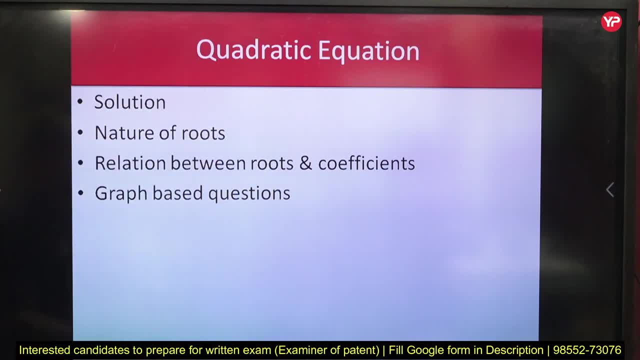 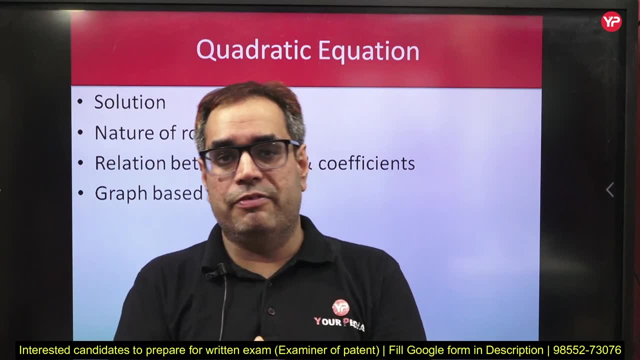 question may be there. and then relation between roots and coefficient. like they give you some quadratic equation and they say that alpha and beta are the roots of this equation, then what is the value of alpha to the power 4 plus beta to the power 4? so this kind of question. 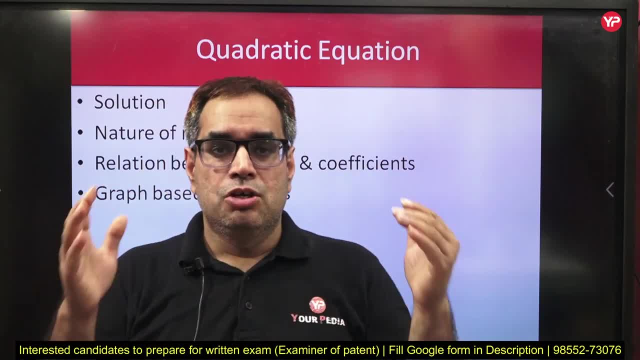 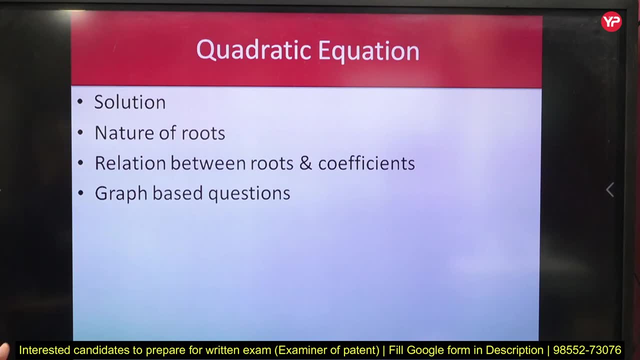 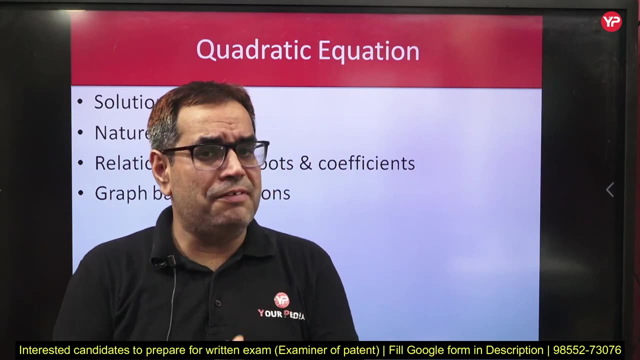 ok, in which we have symmetrical functions of alpha and beta. so these are also important for your exam in elementary mathematics. like: and also you may get questions based on the graphs of parabolas. ok, quadratic polynomials have different graphs, so on the basis of graph. 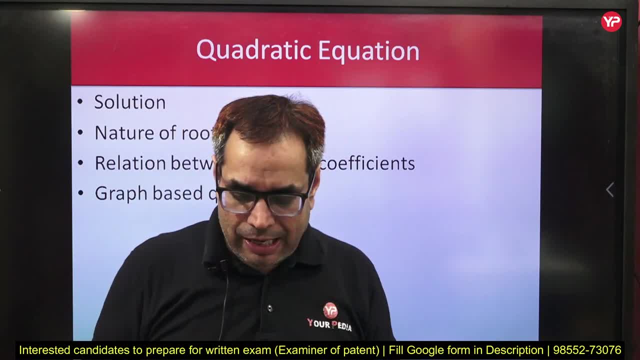 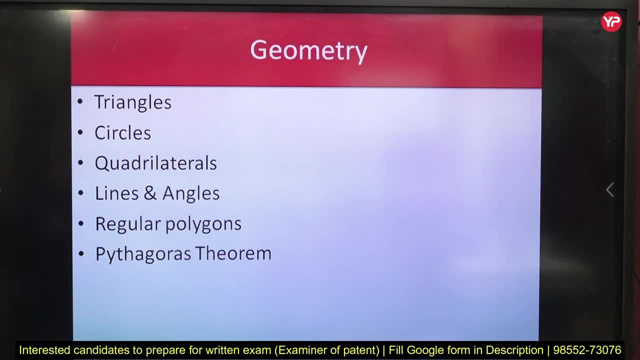 they can form some question. so you have to prepare this and also this may help you in your prelims paper. ok. now what is the next topic? geometry. so geometry is import and ok for your elementary mathematics section. in geometry we have triangles, so you have to prepare types of triangles, different properties of triangles, ok, and then circles, different. 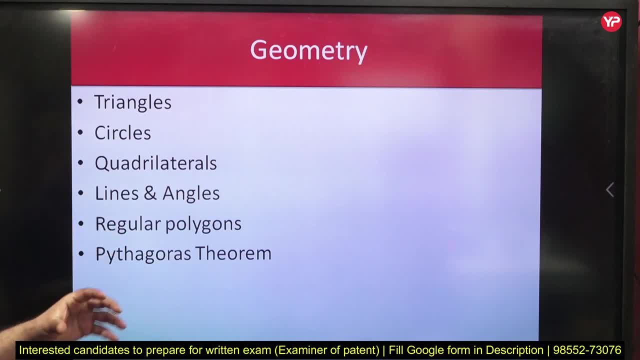 properties of circles, ok. angles, calculation related to different circles, and then quadrilaterals, lines and angles, regular polygons. pythagoras theorem is also very, very important in geometry. ok, so all these topics you have to prepare for your elementary mathematics exam. ok, so that is it for today's lecture. 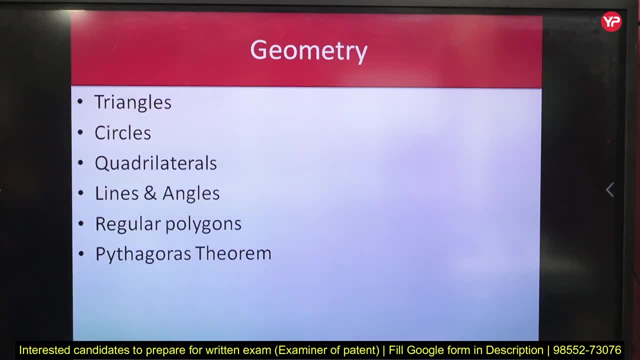 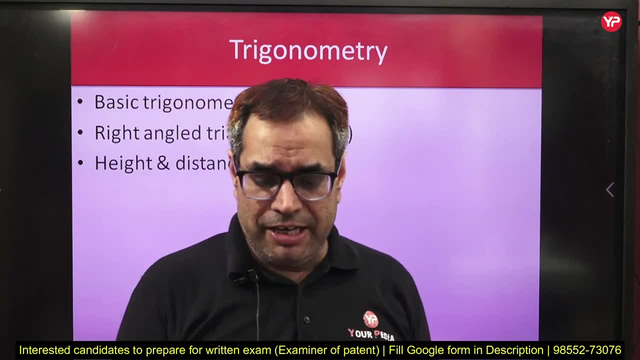 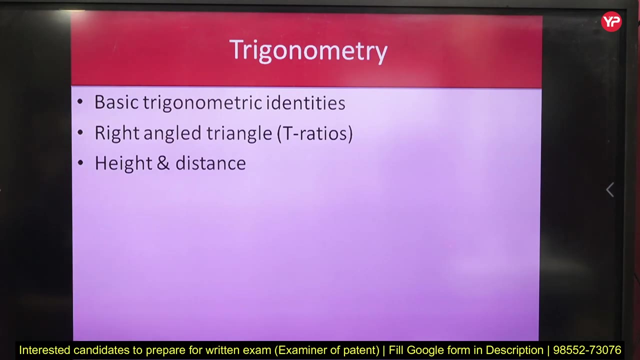 Now let us move to next. so that is trigonometry. 100% trigonometry is important in elementary mathematics and many questions you may get from trigonometry, because always in elementary mathematics questions are asked from trigonometry. ok, so in trigonometry, what we have to cover? 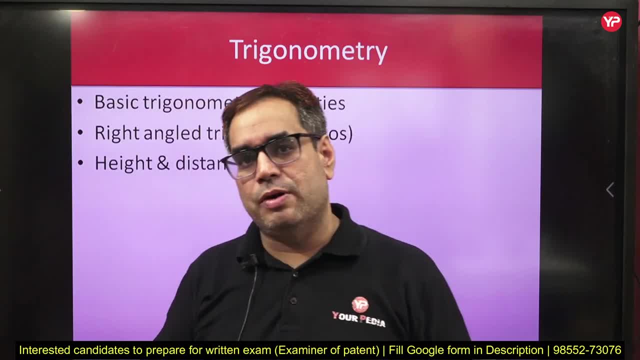 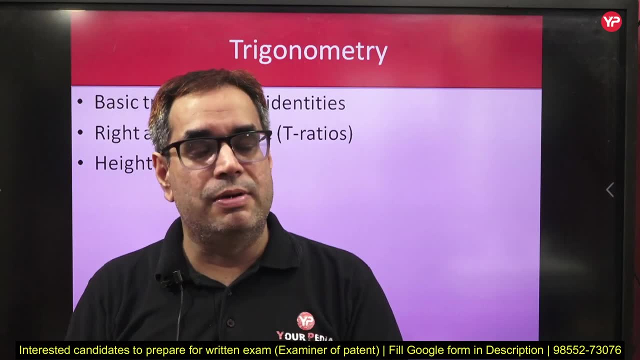 basic trigonometric identities you should remember, like sin square theta plus cos square theta equal to 1. ok, 1 plus sin square theta equal to sec square theta. so we have such many identities. So this is trigonometric identities. you have to remember all those identities and you should 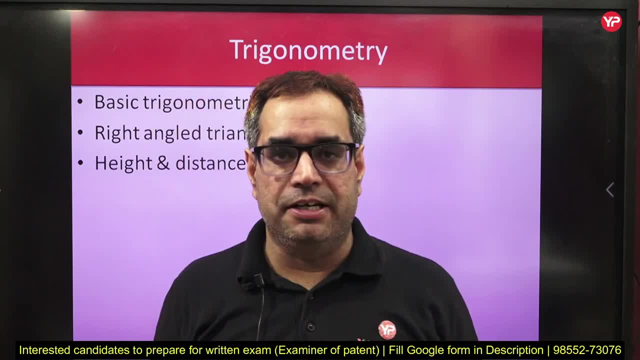 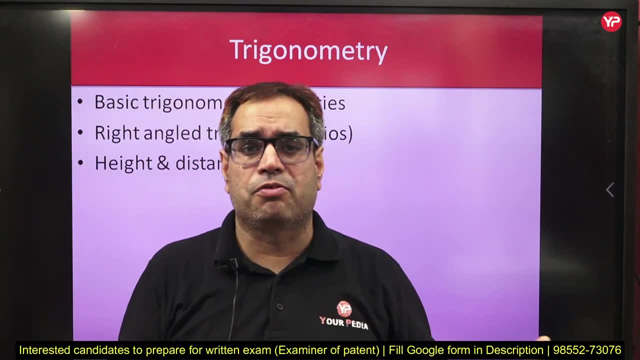 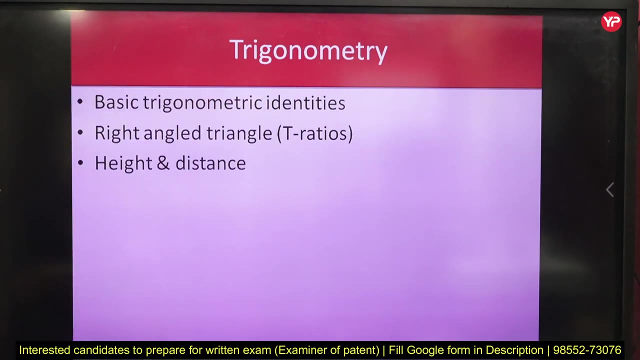 solve questions in which there is use of such identities. ok, you have to do practice for solving different questions, like with our students. we have shared a lot of questions in trigonometry section. ok, so you people have to prepare these all basic identities right now in a right angle triangle. you know, if we have a right angle triangle, we are given. 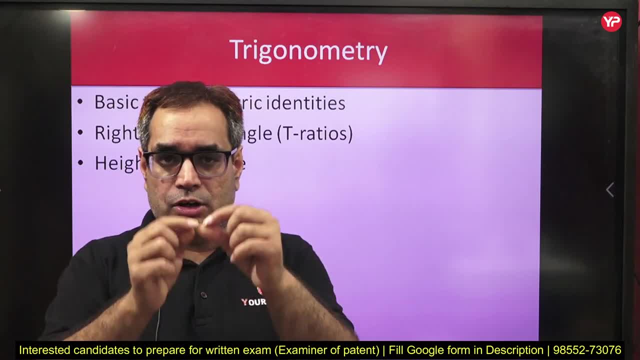 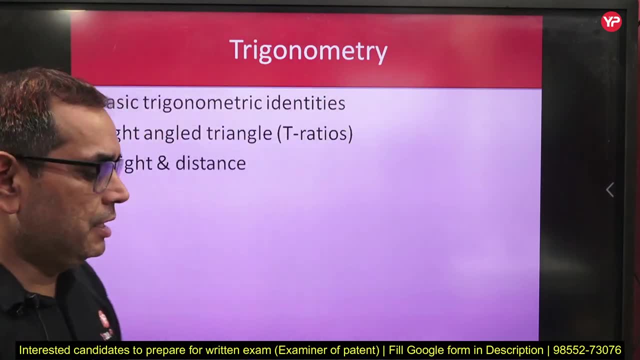 an angle, l theta. It is trigonometric ratios like sin theta, cos theta, sin theta equal to perpendicular upon hypotenuse. so this kind of questions are also important for this exam and then application of trigonometry. that is called height and distance. so compulsorily you may. 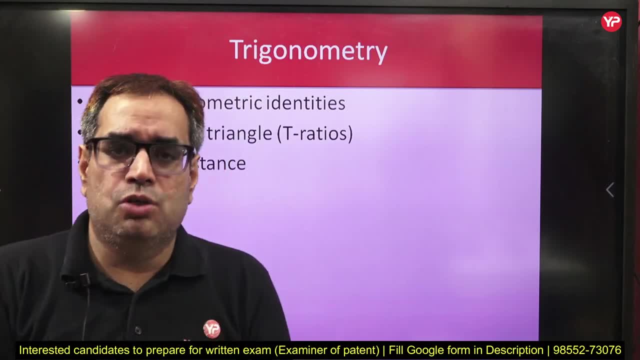 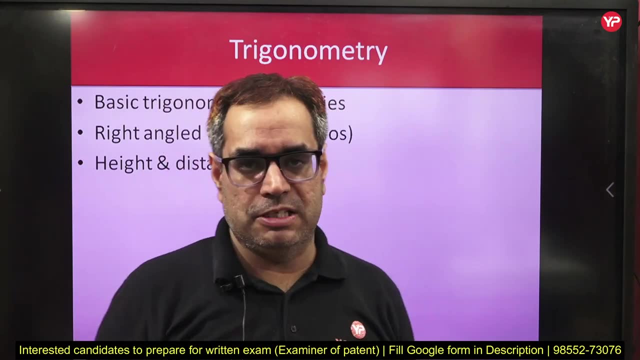 get question from height and distance also, and in prelims also they can ask you question from this height and distance. so you have to prepare this section for your elementary mathematics specifically. ok, now what is the next chapter that you have to prepare? exercise, exercise. 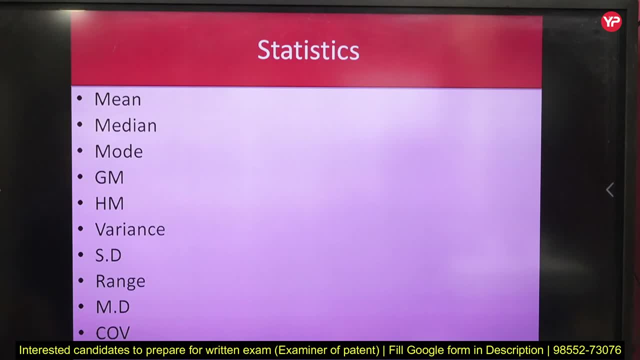 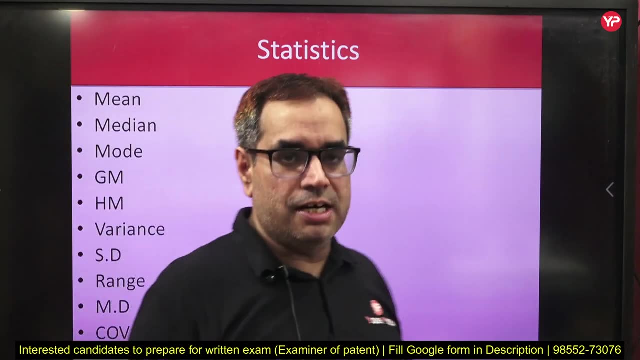 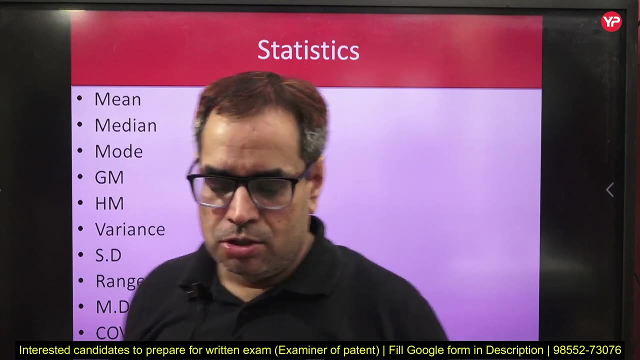 prepare. so come to statistics part right. so statistics is also very, very important in elementary mathematics. in statistics we have different measures of central tendencies, we have different measures of dispersions. so about all of them you should have a basic knowledge like: so mean calculation of mean or average median mode. now you know we have 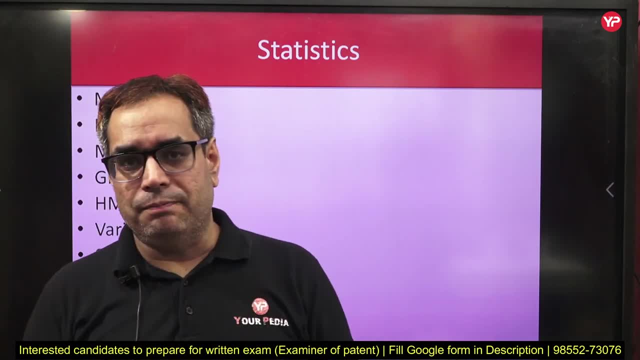 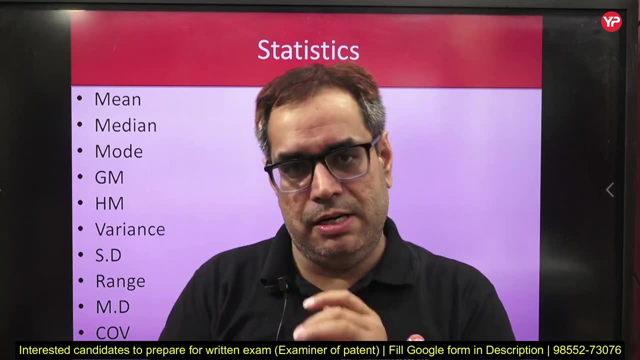 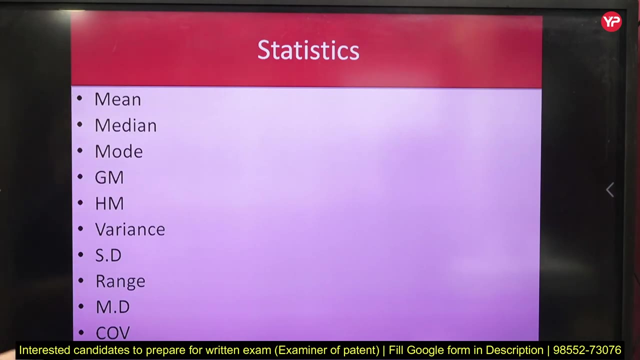 different representations of a data, like we have raw data, we have ungrouped frequency distribution, we have group frequency distribution. so for all the three formats you should remember the formulas, the methods to compute- mean, median and mode. and also what is gm, what is hm, what is the relation between gm, hm am all these things you have to prepare, and then we have 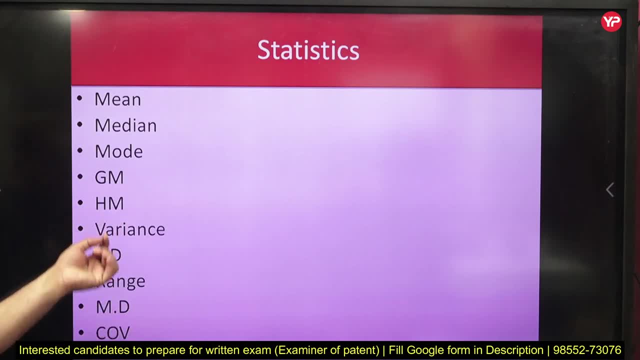 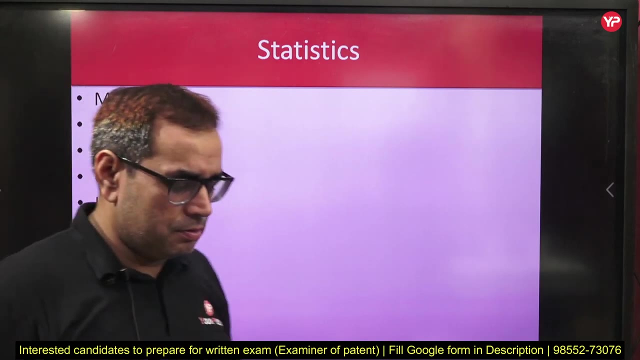 measures of dispersion. these all are measures of dispersion, so you should know how to compute variance of a data set, standard deviation, relation between variance and standard deviation. what is range? what is, what is mean deviation? what is coefficient of variation, cov? ok, so these all are important, your points in the statistics chapter for your elementary mathematics syllabus. you. 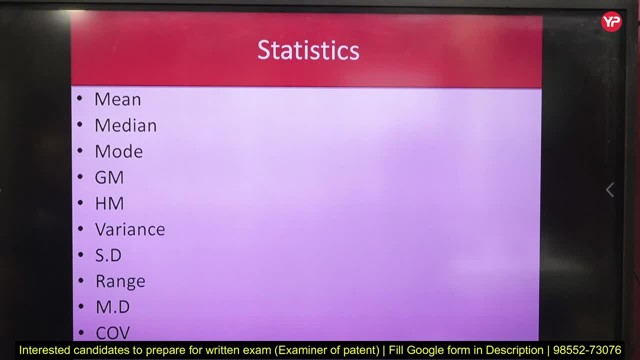 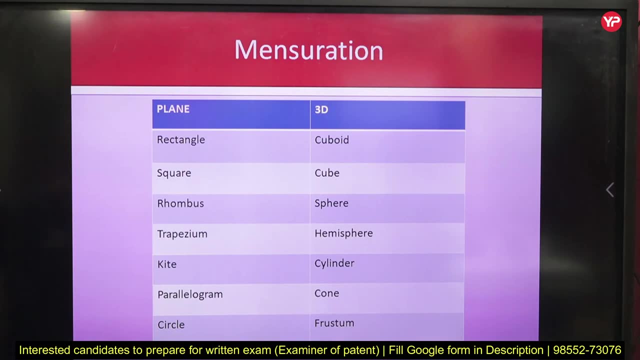 have to prepare these topics. ok, now let us see what is next. so now we have mensuration. you know mensuration is important for both prelims as well as elementary mathematics, strictly ok. so in mensuration we have two sections: one is plane mensuration, another is 3d mensuration. ok, so in plane mensuration we have rectangular square, rhombus trapezium. 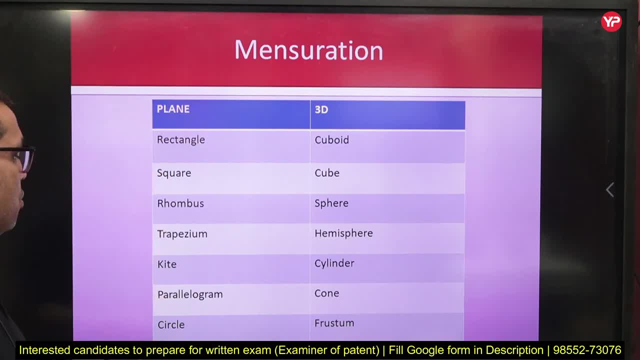 kite parallelogram circle. so you should remember how to calculate the areas of all these things, perimeters of all these things- area and perimeters are important for this- and basic properties. ok, and then we have 3d, like cuboid, cube sphere, hemisphere, cylinder, cone, frustum, all this. 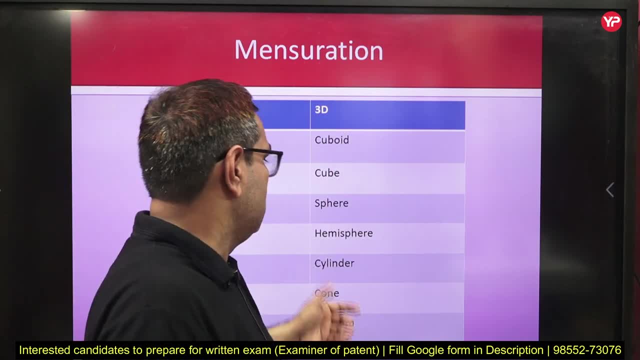 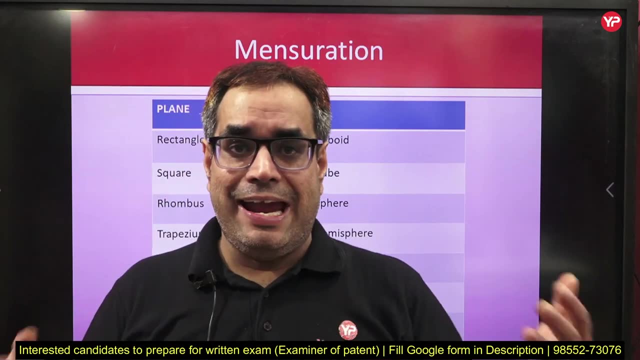 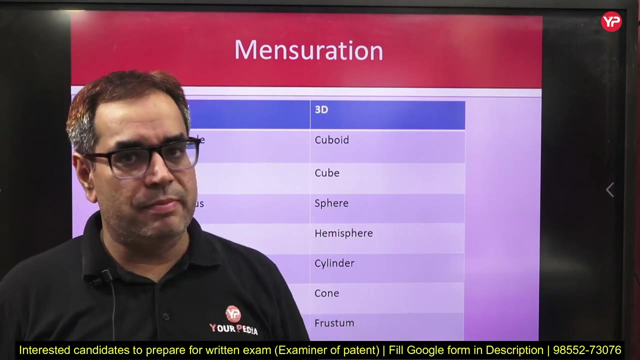 so in in this right corner, right corner, all these are parameters, very important because, column, we should remember formulas to compute the surface area, curved surface area, total surface area and volume. so this is also important. many questions you may get from this menstruation part in your elementary mathematics paper as well as in aptitude section also. they can. 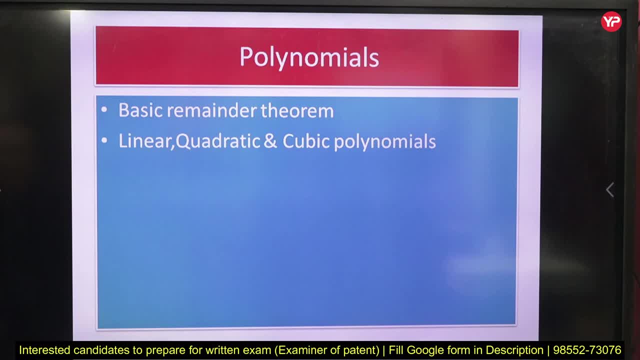 ask you questions from these topics. ok, now we have polynomial, so polynomial is also important for elementary mathematics paper. in polynomials there is one remainder theorem that you should know and different properties of linear polynomial, quadratic polynomial and cubic polynomial. ok, you need not to go beyond cubic up to cubic you have to prepare, and also relation between 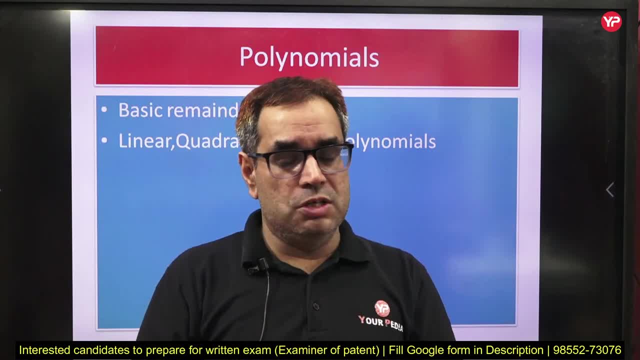 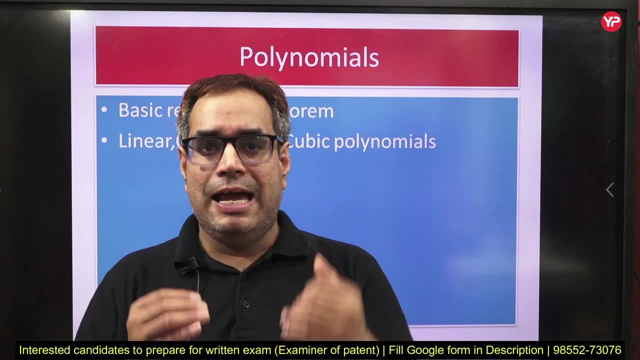 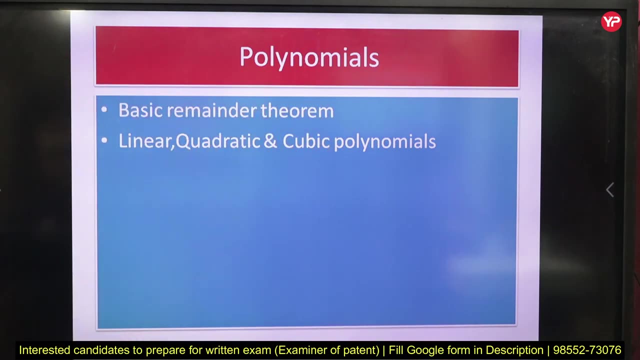 roots and coefficients of a polynomial. ok, so those formulas you should understand and you may get question from that. factorization of polynomials is also important. fcf, lcm of polynomials is also important. so these are the formulas that you should understand and also important so that also to be prepared right now let us move to the next section. 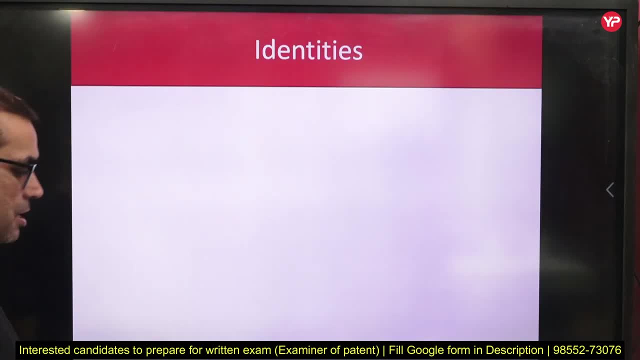 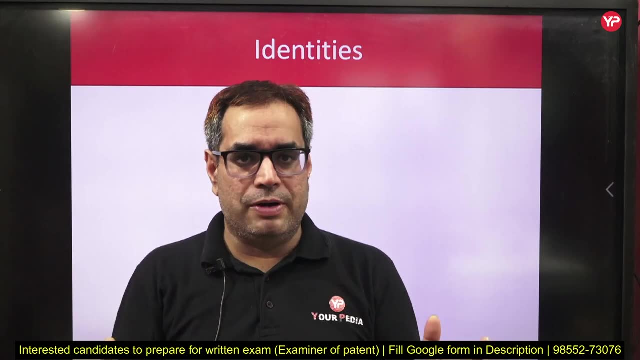 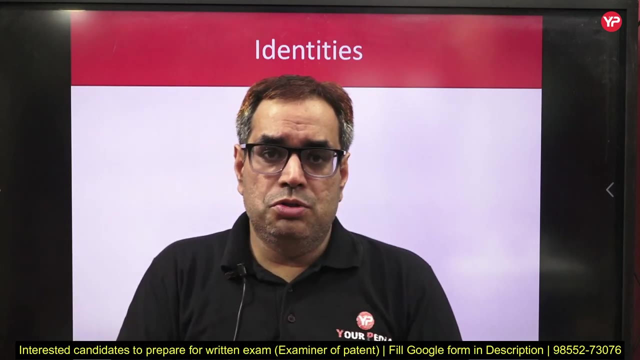 so that is identities. you know we have different identities, so you should remember all the formulas like a plus b whole square equal to a minus b whole square. equal to a cube plus b cube- all these identities. there may be some questions in which we may require to use some identity. ok, so once we prepare, we remember all the identities and we solve. 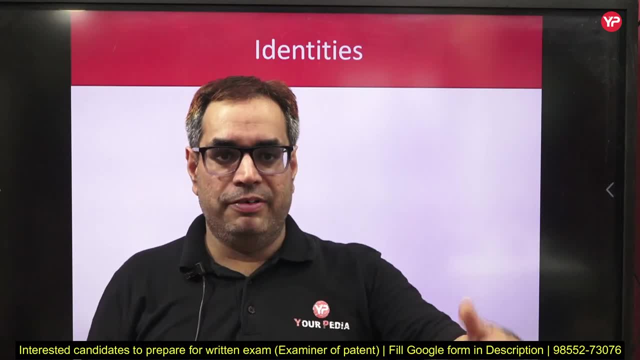 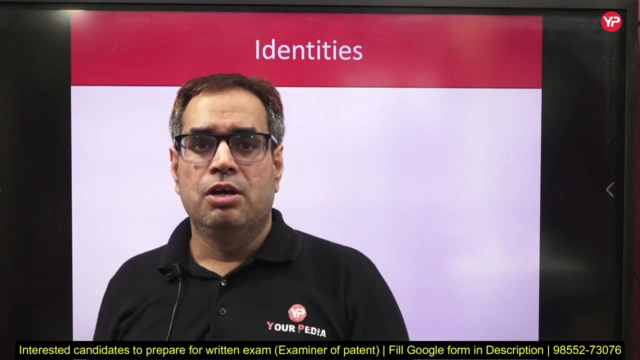 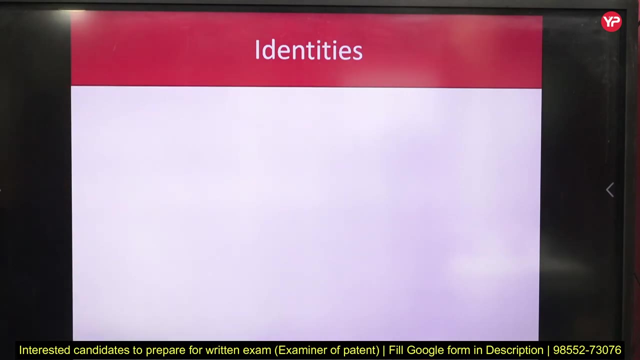 some questions, then only we can apply them in the question we randomly get in exam. ok, so you have to remember all the identities also and you have to solve some questions in which we need identities, right then? what is the next next topic? so it is sequences and series. ok, so 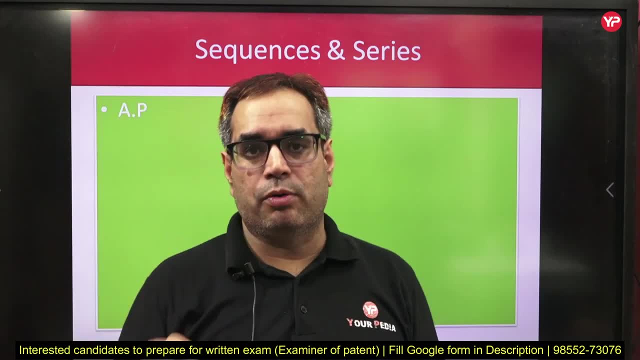 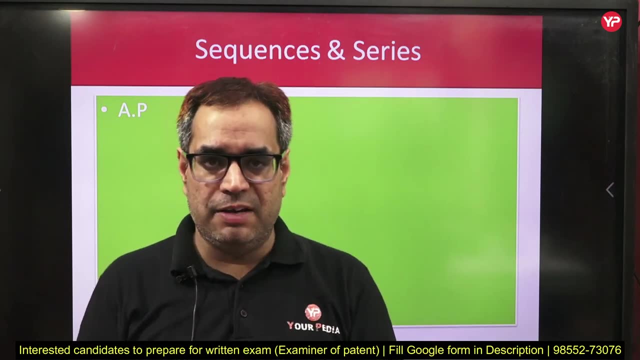 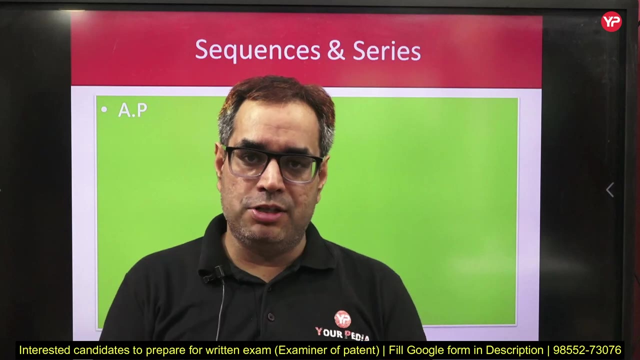 in sequences and series. you should prepare arithmetic progression ok: how to find the nth term of a ap, how to find the sum of n terms of an arithmetic progression, and there may be some questions based on the properties of arithmetic progression. so you should know all the basic properties of arithmetic progression, right. 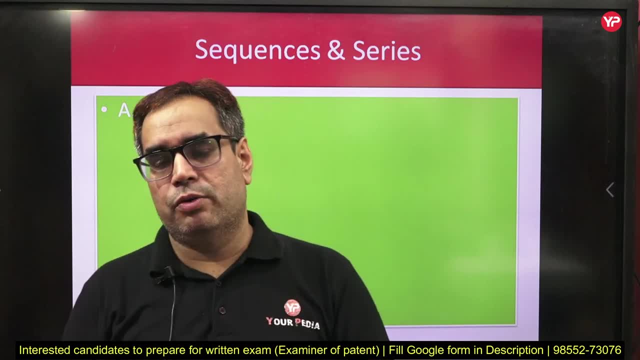 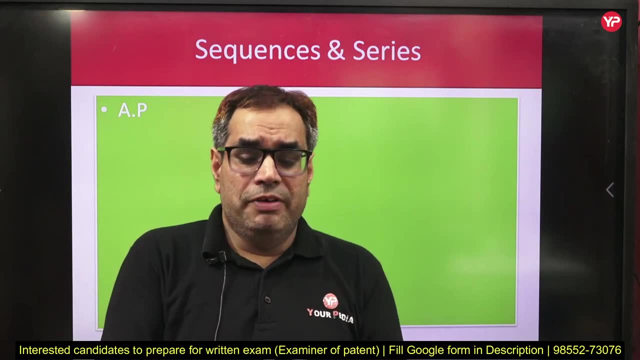 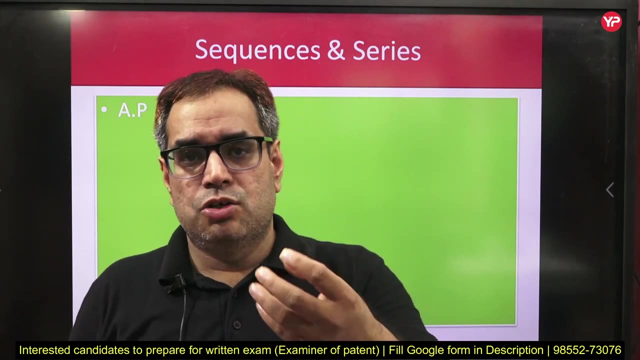 and also there is some difference method. ok. so this year also they ask one question to find the nth term of some sequence that was an ap, so in which the consecutive difference, the difference of consecutive terms, was in ap. ok. so difference method is also important in sequences, ok. 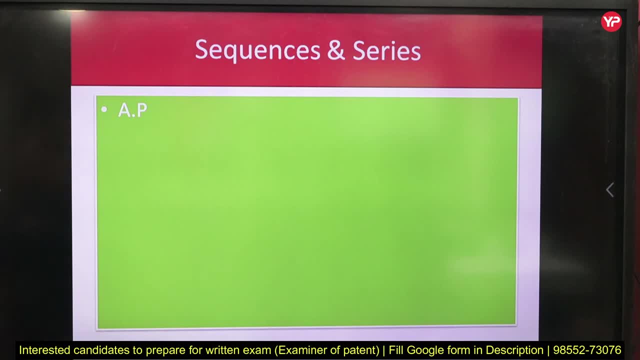 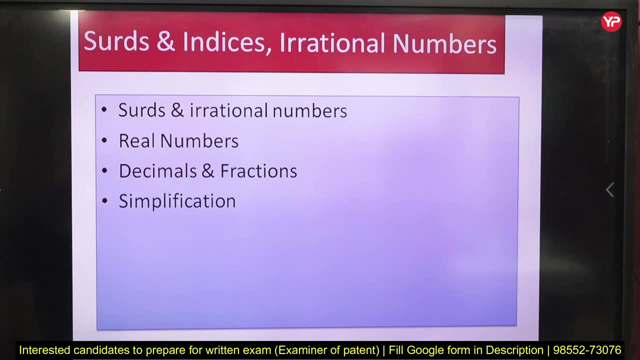 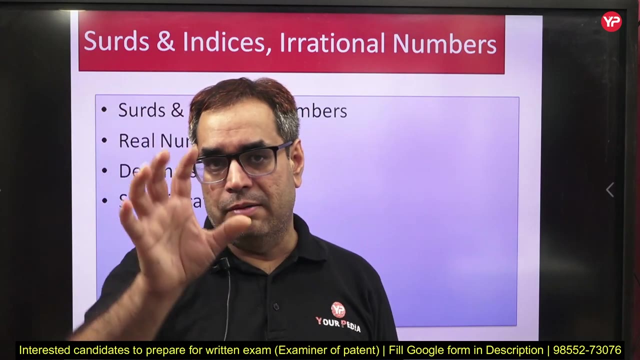 you have to prepare that right now. let us move to next part, that is surds. indices erase irrational numbers, so this is also useful in your elementary mathematics section. so questions may be there based on square roots of a number of a surd. you should have a practice. 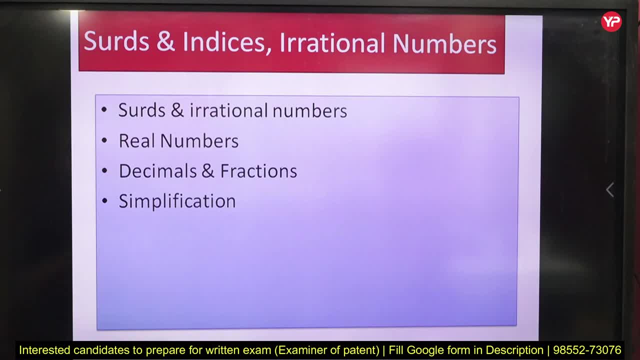 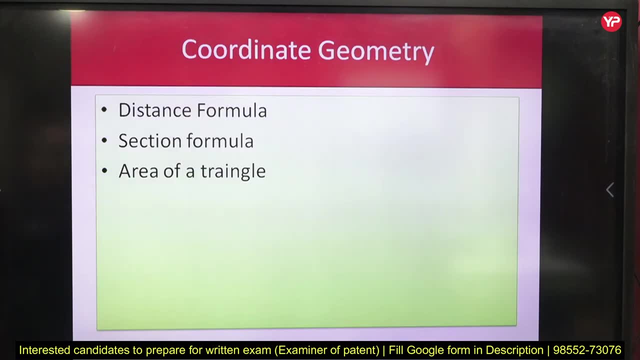 of that real number, properties, decimals and fractions, simplification, all these basic topics you should prepare. ok, now we have coordinate geometry. ok, now we have coordinate geometry. ok, so in our syllabus coordinate geometry is also. you may get question from coordinate geometry also. right, in coordinate geometry we have to remember that the section formula 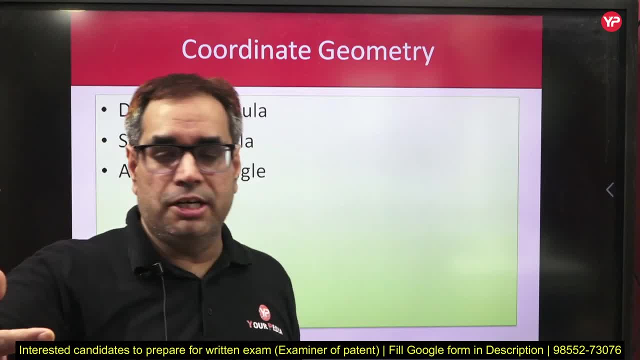 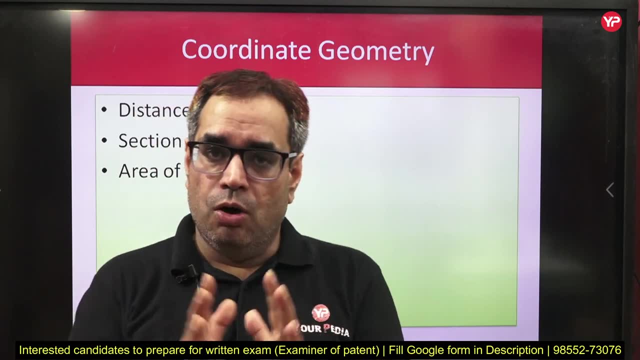 and are of a triangle. ok, as you know, you need to know to go into the details of other curves like parabolas, aliases, hyperbolas, circles. do not go in to the details of those only. this thing is important for the your elementary mathematic section in coordinate geometry. 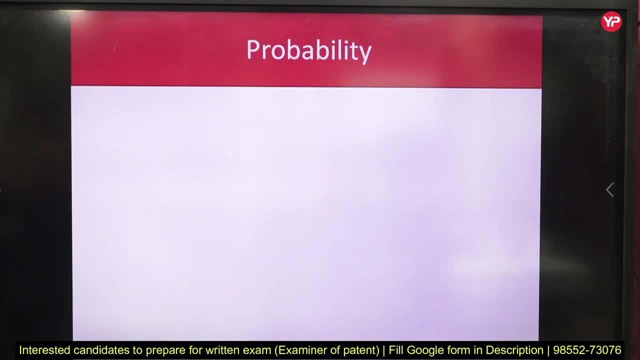 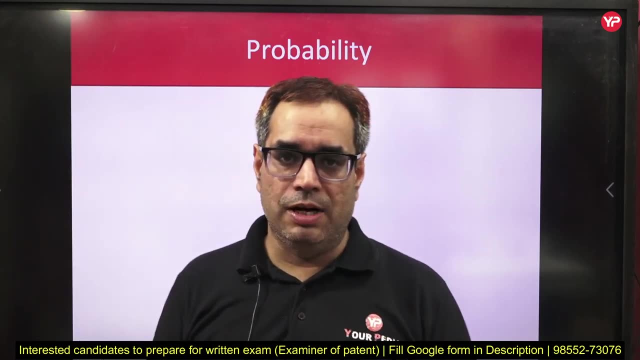 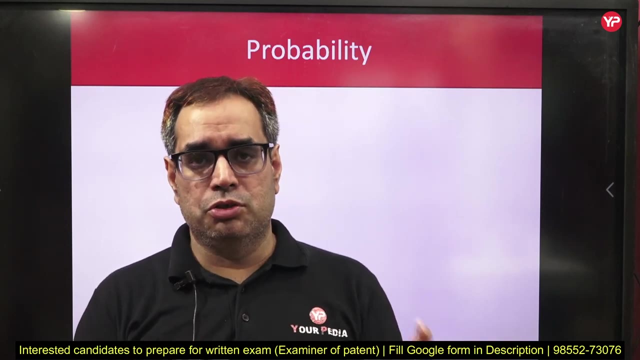 right. and then we have probability. yes, probability is also important for prelims as well as for elementary mathematics section. in probability, the most common formula, probability of an event equal to favorable number of cases divided by total number of cases. in most of the questions this is used, so you should know how to use this. you should solve different variety of. 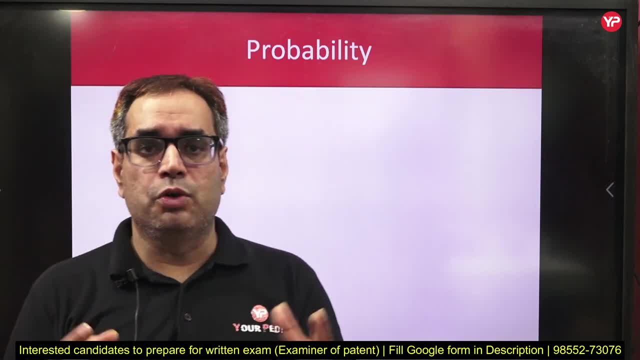 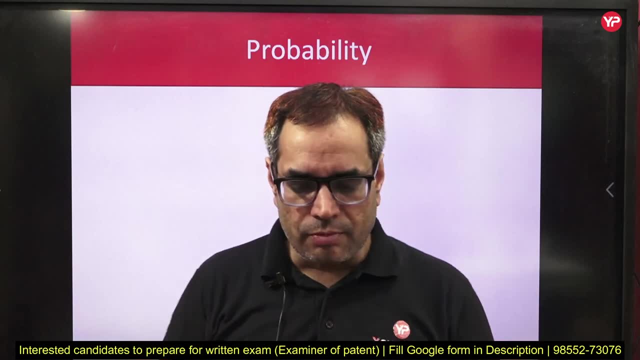 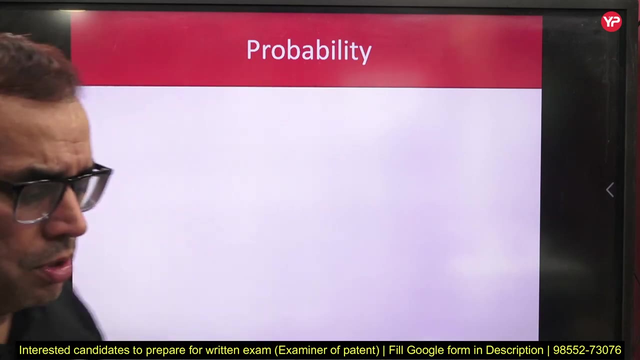 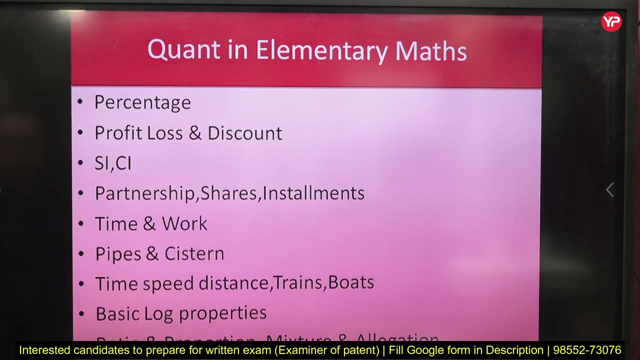 questions and then some basic relationship between two events like A union B, A intersection B. you should know. so such questions may be there in your exam. you have to prepare probability in both elementary mathematics as well as for your prelims examination. now come to next topic, that is. so let us have a look here. these topics generally we study in aptitude section. 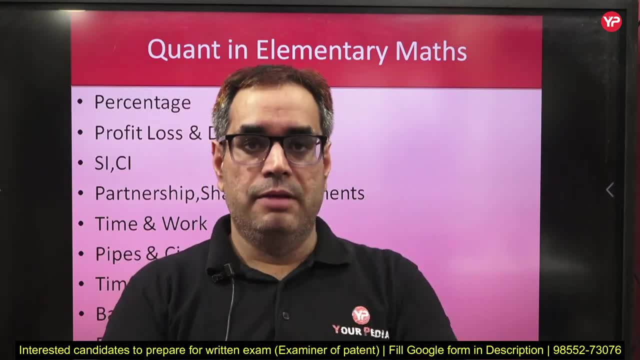 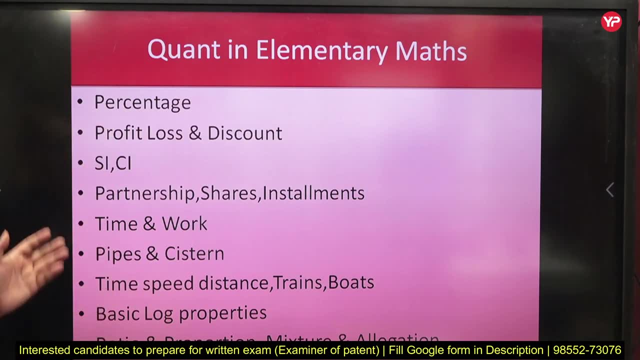 which may be asked in elementary mathematics paper. also, remember you may get question from percentage, from profit, los and discount, from simple interest, compound interest, partnership shares, install time at work time, speed distance boards, trains, basic log properties, logarithm properties. then we have ratio and proportion, mixture and allegation. so these are main topics for 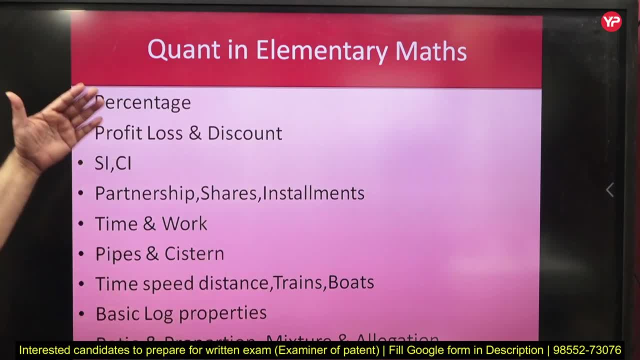 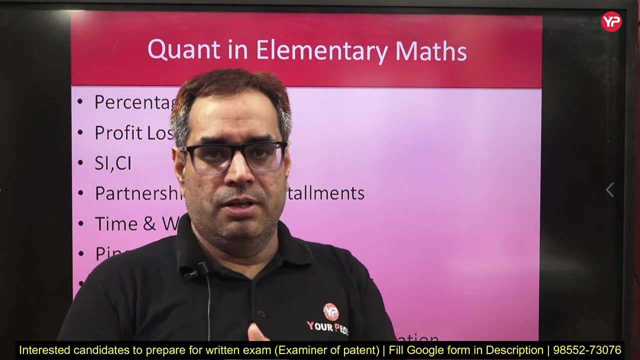 prelims examination strictly. you have to prepare all these topics for your prelims examination, most important topics for your prelims examination and also, so there is a possibility that you may get question from these topics in elementary mathematics also. ok, most probably, most probably other topics which i have discussed up to now: those 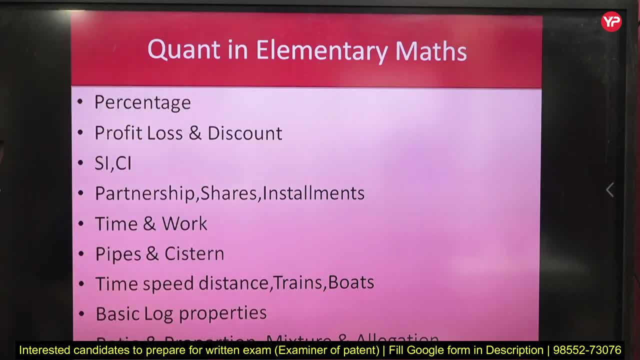 are considered in elementary mathematics. but they can ask you questions from these topics also in your elementary mathematics paper. so please keep revising after the prelims also, you have to revise all these topics in prelims. these are 100% sure topics because in previously conducted examination also, majority of the questions they asked have feedback. 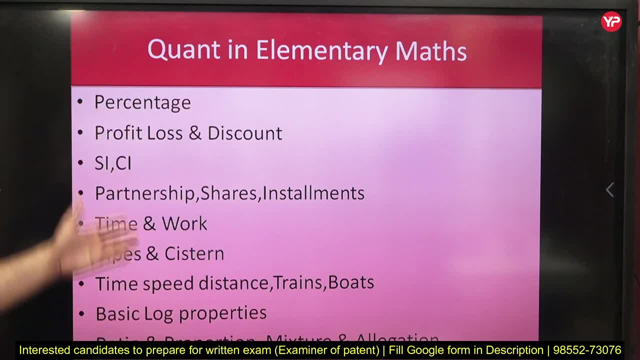 provided by the students. majority of the question was from these topics. so again, for prelims, you have to prepare these topics, and also for elementary mathematics, you have to keep in mind that these questions may be there right. so now i hope that you have got detailed idea about the syllabus of your elementary mathematics paper. ok.